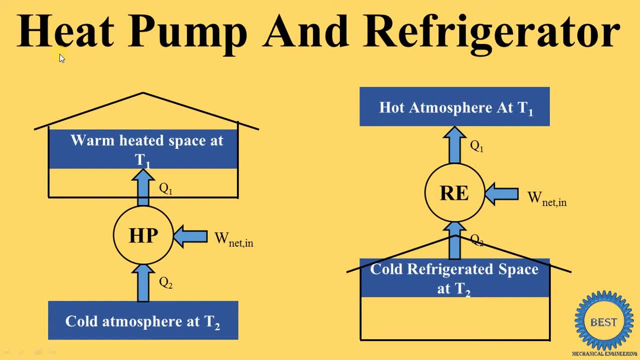 heat pump is required to increase the temperature of the heat pump, The room or a certain spaces means it is used for the heating purpose. And what is the functions of refrigerators? So in India we use the refrigerators and AC for the cooling purpose. 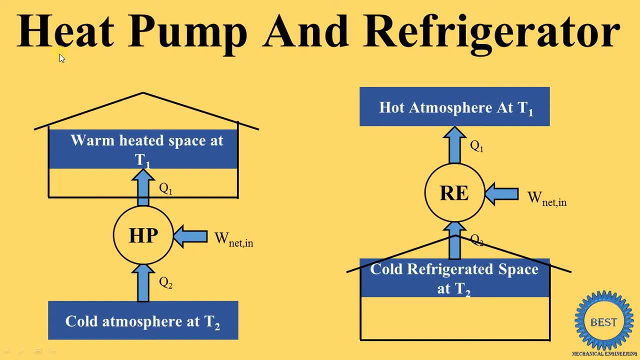 So we use the AC for cooling of the our rooms and we use the refrigerators for cooling of the waters: cooling of the vegetables, medicine, fruits and water. So this is the basic functions of the heat pump and refrigerators. Heat pump is used for the heating purpose. Refrigerator. 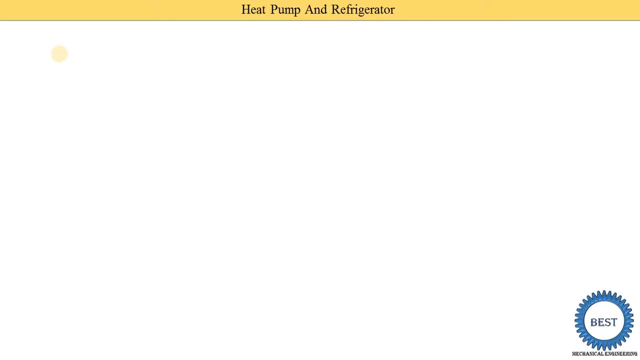 is used for the cooling. So now we understand what is the heat pump. Heat pump is a thermodynamic system operating in a cycle. So here again the cycle word is used means in a heat pump there is a number of processes going on And what the heat pump is do Heat pump is absorb heat from the low. 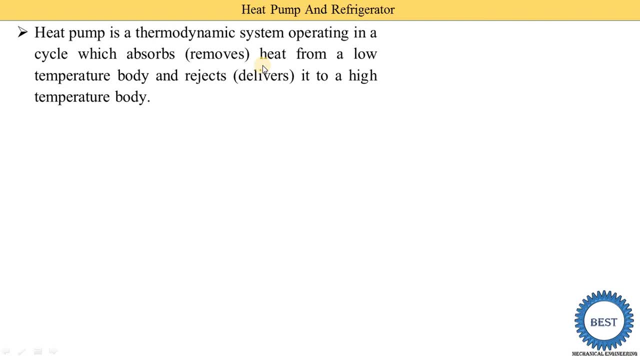 temperature body and reject it to the higher temperature body. Now let we understand these words. So here we are using these diagrams. So here you see, this is the heat pump. In a heat pump we supply some work done. that is the W net inch Generally, the heat pump and refrigerators. 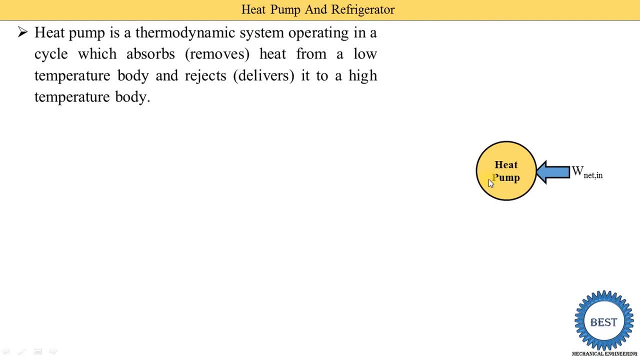 are work consuming device. In the last video we study about the heat engine. So heat engine is the work producing device means they produce the work, But here the heat pump and refrigerators are consuming the work And when we supply this work done to the heat pump, they produce. 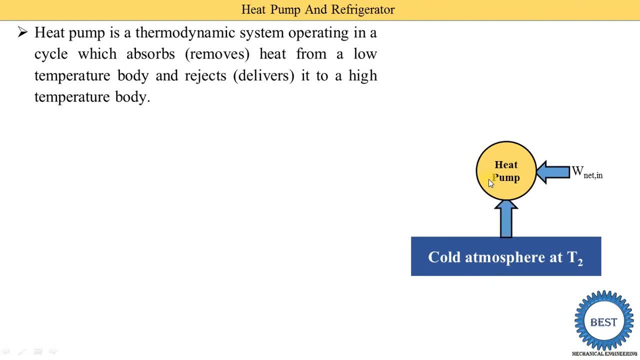 more work, But now we need to think about the power equipment also. that is heal what we are saying. So then, what do you say? that this heat pump is used to run the machine, to generate electricity. OK, so here we mention: absorb the heat from the colder atmosphere's. Okay, so here we mention: absorb the heat from the low temperature. 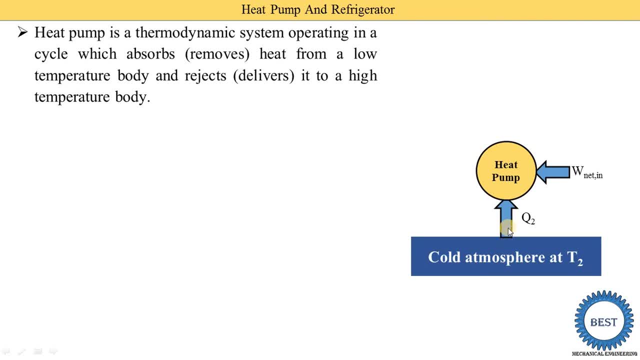 body. So here this is the low temperature body, Or we mentioned that it is a coal temperature. higher temperature is there? okay, so here we absorb the q2 quantity of the heat. okay, so in a different book the different notation is given, but generally we use the two terms of the sink portions and the 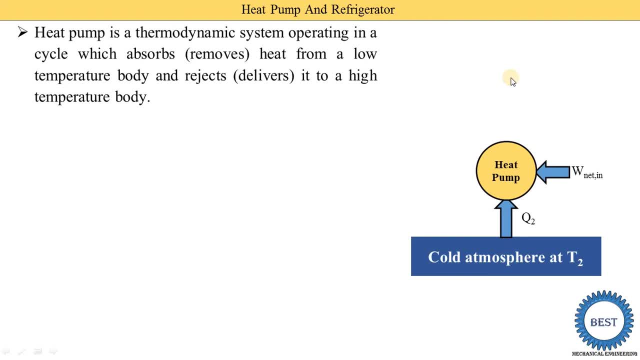 for the source function, we use the one for the heat engine, heat pump and refrigerator. so these things are not make any confusions in our minds. okay, now at the upper part, in a source that is a warm, heated space at a temperature t1s because we require the heating. okay, so heat pump is used for. 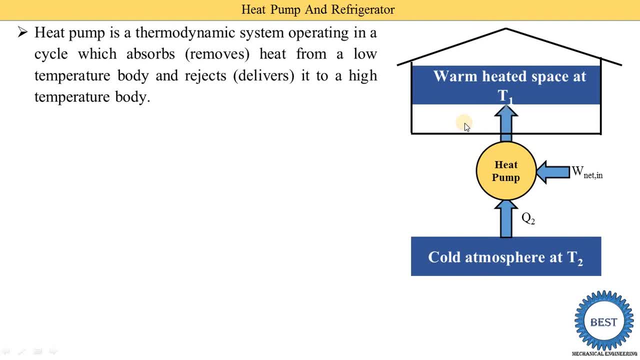 the heating purpose. okay, so here our output is there. okay, so this heat pump is reject the heat energy to the hour room or a space, and the quantity of the heat energy is the q1. okay, so here we see that the q1 is equal to q2 plus w, because here you see, that is the two things are. 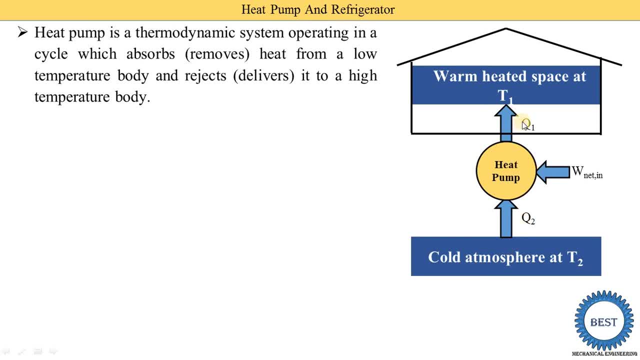 supplied to the heat pump, this and q2 quantity of e. so q1 is equal to q2, q2 plus w net. okay, so our room is heated by using this heat pump and this heat pump is absorbed. the heat from the cold atmosphere means heat pump is absorbed. the heat from the outside atmospheres 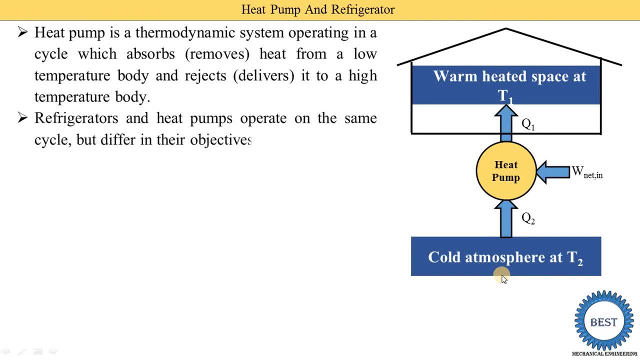 now refrigerators and heat pump are operate on the same cycles means in a single component we are able to convert the refrigerator in a heat pump or a heat pump in a refrigerator. okay, so that means they are operate on a same cycle but different in their objectives. okay, so their. 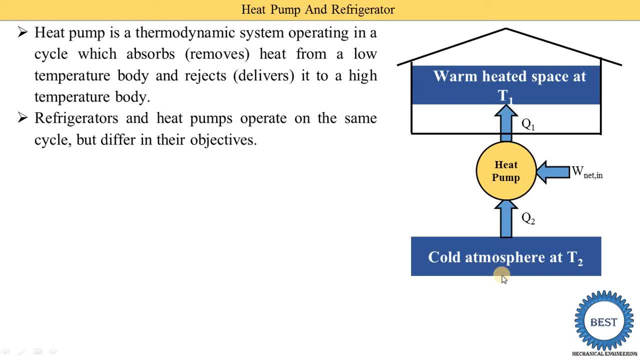 objectives are clear, because we earlier already explained: heat pump is used for heating purpose, refrigerator is used for the cooling purpose. this is the basic objective. the objective of a heat pump is to maintain the heated space, and in india we are not using the heat pump. okay, so at a higher. 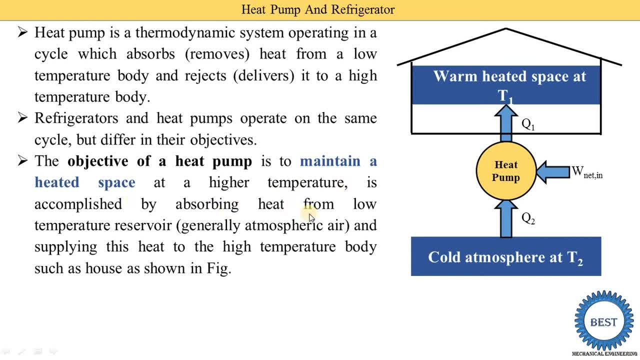 temperatures is accomplished by absorbing the heat from the low temperature reservoirs, so generally it is the atmosphere air. so this cold atmosphere at the t2 is our atmosphere air. okay means it is outside area of the our home or a room that is over the cold atmospheres and they absorb the heat q2 quantity and supplying this. 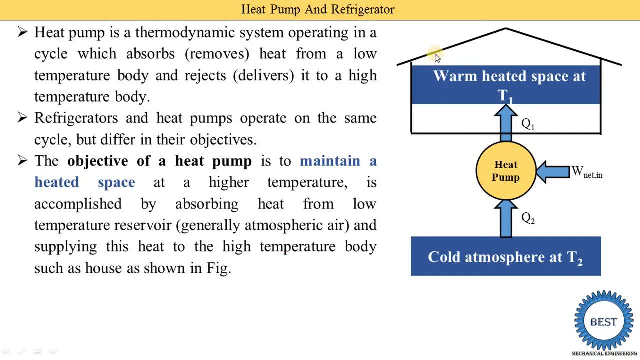 heat to the higher temperature body, such as the house, as shown in this figure. okay, so here you see. this is our house. so in a house, we supplied the heat energy and our house temperature, or a room temperature, is increased. now, before moving ahead on the objective of a refrigerator, i request: 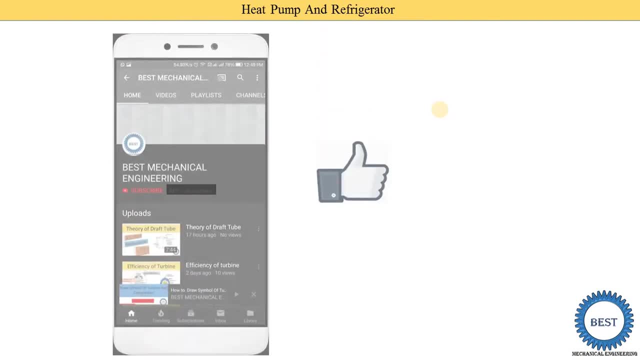 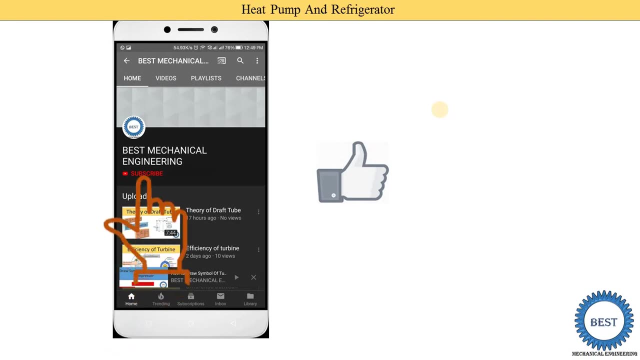 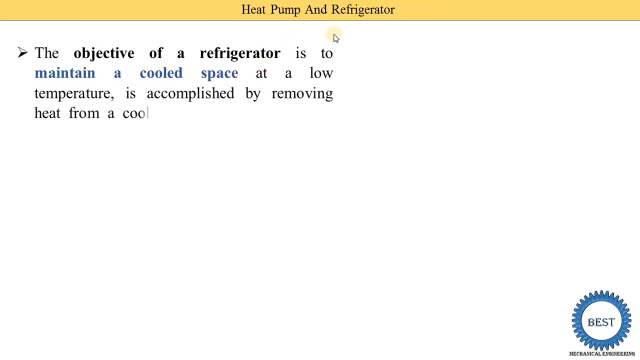 you to subscribe my channel for watching the more video related to the engineering, thermodynamics and other subject of the mechanical engineering. for engineering, thermodynamics and bme subject, various link is provided in descriptions for other subject. i request to visit the playlist now. next, we understand the objective of refrigerators. the objective of refrigerator is to maintain a 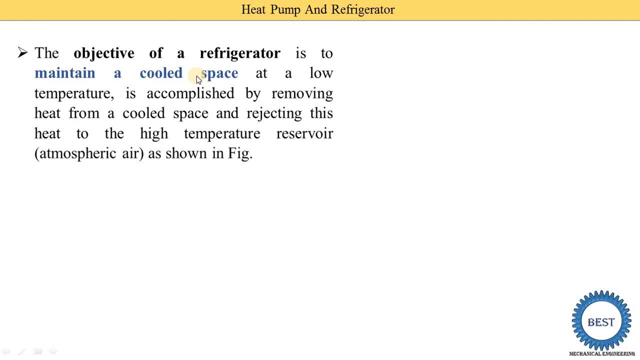 cool space at our home, we use the freeze. okay, so this is also known as the refrigerators. okay, why we use the refrigerators? to maintain the cool space, to maintain the cool vegetables, waters and different fruits and vegetables, as well as the medicines. okay, so we maintain the cool space at a lower temperatures is accomplished by removing heat. 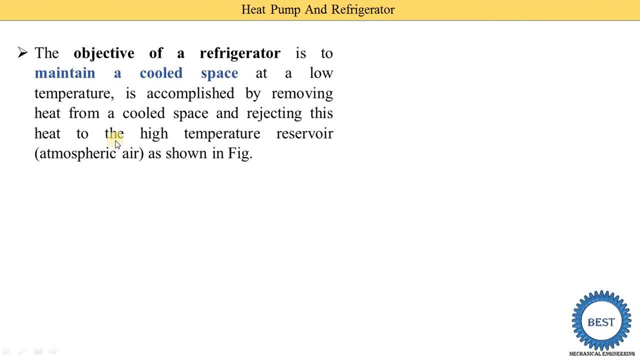 from a cold space and rejecting this heat to the higher temperature reservoirs. and higher temperature reservoir means it is the atmosphere, as shown in these figures. so our refrigerator temperature is reduced. how this temperature is reduced? because the heat energy inside this refrigerator are absorbed by the one gas it is called as the refrigerators, and this heat energy. 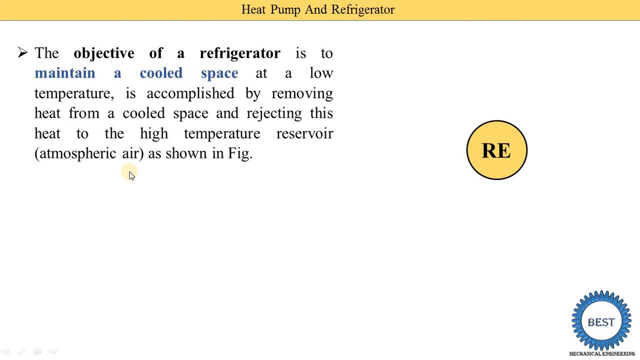 is rejected to the outsides. okay, so on the one side of the freeze you check that the one side of the freeze temperature is the higher. okay, that is called as the condenser. so this heat energy is rejected to the outside, to the refrigerators. now, here you see. this is the refrigerators. 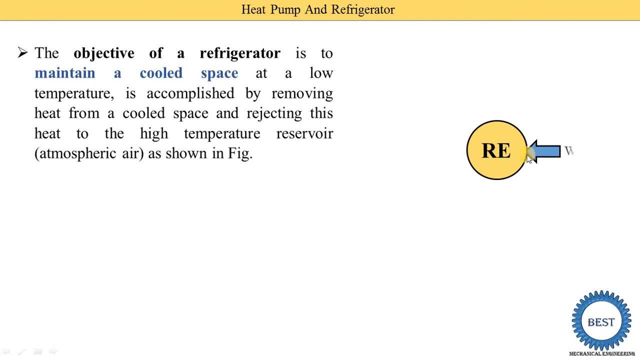 in which we supplied some work done, because it is the consuming devices we supply w net and this refrigerator is absorbed, the heat energy from which they absorb the heat energy from the cold refrigerated space at the temperature t2. okay, so this refrigerator is absorbed the heat and the quantity is the q2. same way at the lower portion. 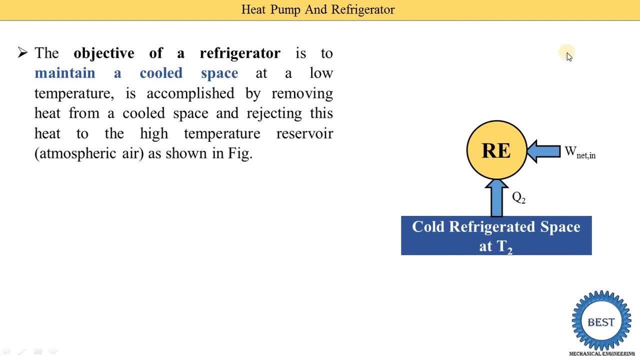 means for the sink we use the two terms and for the upper portion we use the one terms. okay, for the same, all the three cases like heat engine, heat pump and refrigerators, and here in a refrigerators, our room or a space in a bottom portion, because refrigerator function is to. 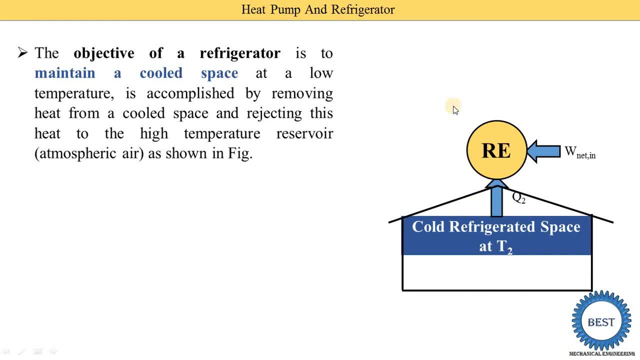 reduce the temperature means: here our output is there and in a heat pump our output in the source portions. okay, so this further heat energy is rejected to the hot temperatures at the t2 and our hot temperature is our atmospheric air. okay, both heat pump and refrigerators are the what. 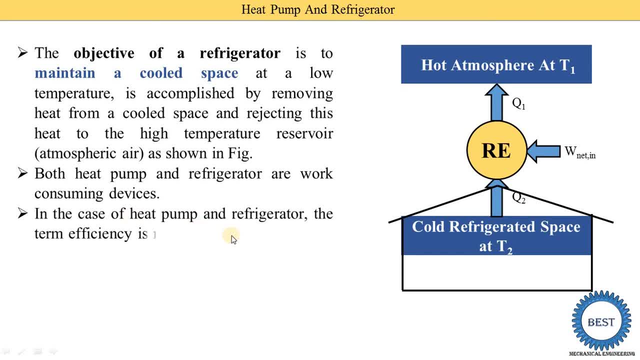 is that we already discussed. in this case of a heat pump and refrigerator, the term efficiency is replaced by the coefficient of performance. okay, so here the coefficient of performance. what is used? instance of the efficiency. so in a heat engine we find out the efficiency, okay, but in a heat pump and 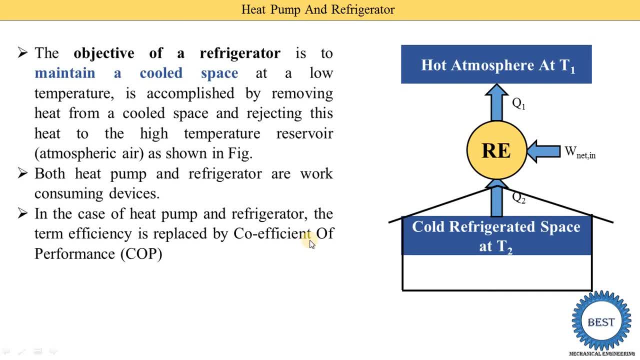 refrigerator. we are not find out the efficiency, but we are find out the cop. the full form of cop is the coefficient of performance. for that we need to understand the three terms. first one is the q1. q1 is the heat rejected by a system in a kilojoule. so here you see this: q1 is the heat rejected. that. 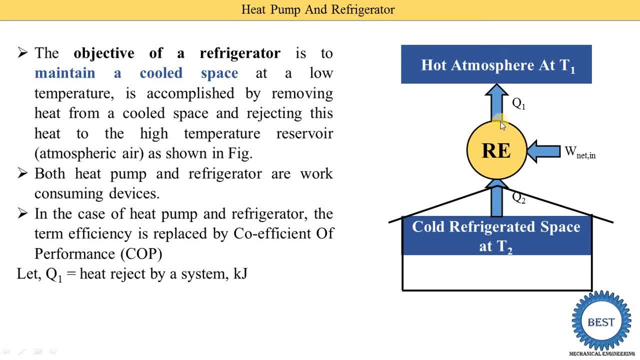 is going in an outside arrow. okay, this is the refrigerator, or either a heat pump is there. so q1 is going outside from the refrigerator or a heat pump. that's why it is called, as the heat is reject. qt is the heat absorbed by the system. so here you see: refrigerator is absorbed, the heats. 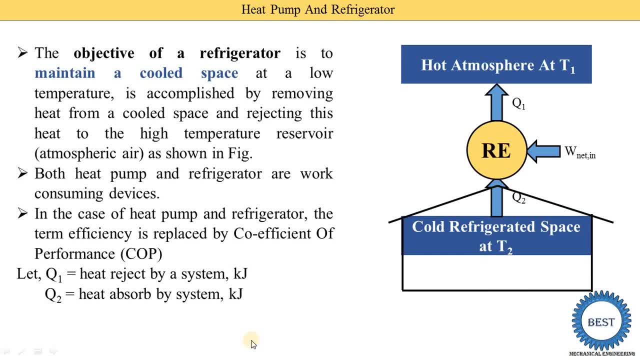 means arrow is coming inside the refrigerator or a heat pump. okay, unit is same. that is in the kilojoule. next is w net. that is a network input to the system. in kilojoule means we need to supply some work then okay. so there is a three main parameter. is that q1, q2 and w nets? now we know the first law of the. 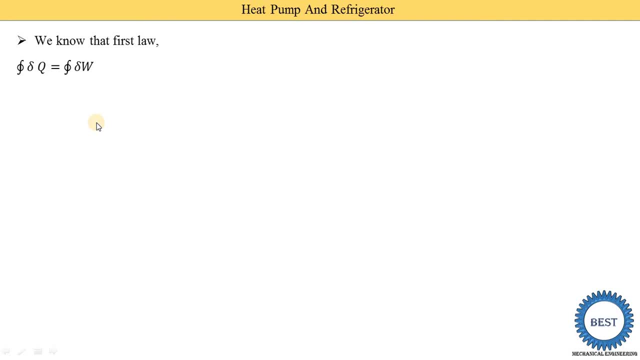 thermodynamics. first law of thermodynamics means it is applied for the cyclic process. okay, when the cyclic process is there, at that time the cyclic integrations of heat energy is equal to scientific integrations of work energy. okay, so in a heat pump and refrigerator there is a two heat. 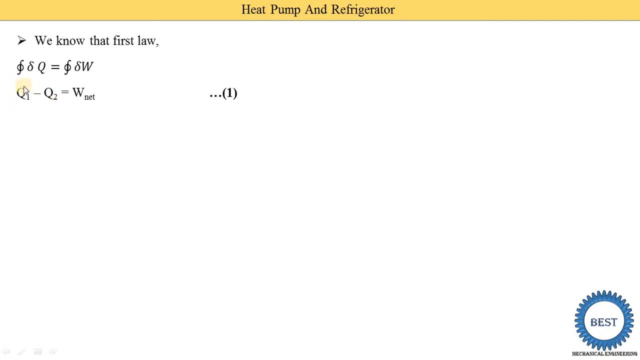 interaction is that. that is a q1 and q2- okay, so we know that the q1 is higher, that i already discussed. so q1 minus q2 is equal to w net. that is only one work interaction is there? okay, the cop of heat pump and refrigerator can be find out as or can be defined as, so cop is equal to desire. 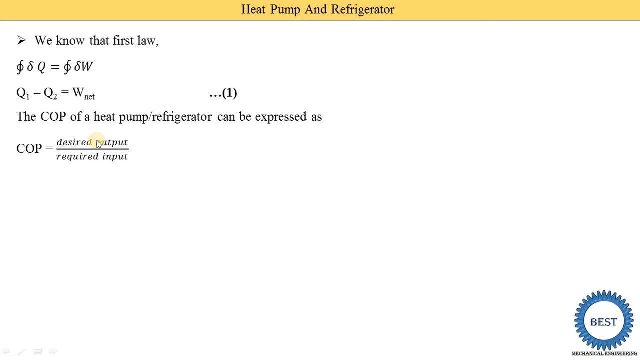 output upon required inputs means equation of the cop is same as the efficiency, that is, output upon input. okay, but why the cop is used? for that i make the one different video. what is the different between efficiency and cop? what is different? the video of the cop and efficiency. i provide these. 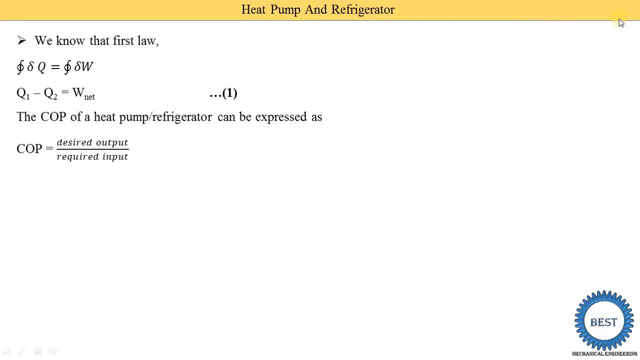 links in a card card, mean on a top right screen of your mobile or laptop, you see the i symbols now. so first we find out the cop of heat pump. so here you see this, the diagrams of the heat pump. okay, so in this diagram, so one thing is clear: what is the input? our input is the w net, but what is? 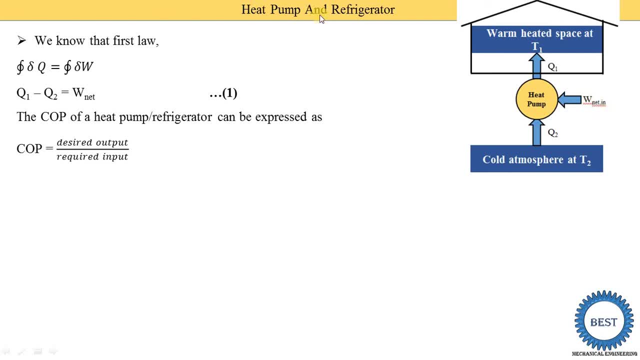 the output, okay so in a pump and refrigerator, lots of students are do that so. in a pump and refrigerator, lots of students are do that. so in a pump and refrigerator, lots of mistake that they are not know why. which side is our output is there, okay, so 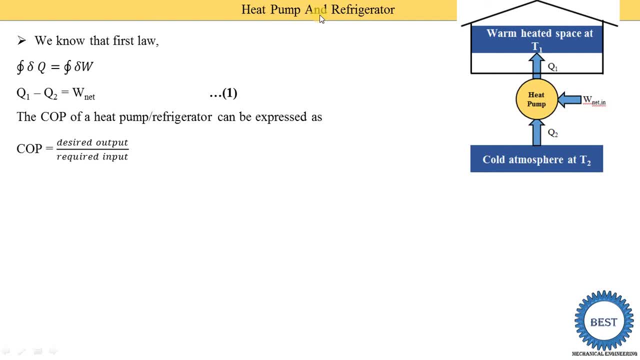 output in a heat pump. so functions of the heat pump. is the heating? okay, so where the heating is done, heating is done near the source. okay, so our higher temperature is our output. okay, because we require the heating. okay, so here our q1 is the output. okay. so equations of the COP for the heat pump: COP bracket. 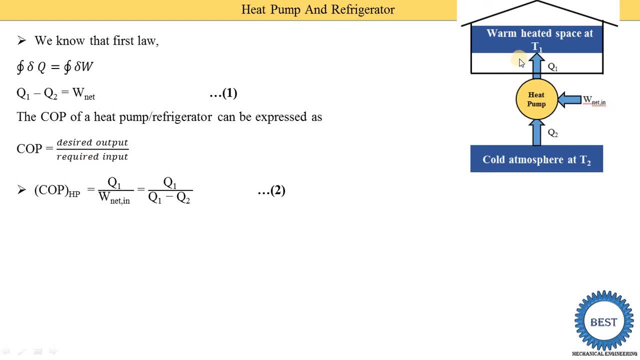 over HP is written, that is for the heat pump: okay, desire output is the q1, because here the higher temperature is there. divided by: require work input, require what input is the W nets? okay, and W net also written as the q1 minus q2. from these equations, from this equation 1, here you see, W net is equal. 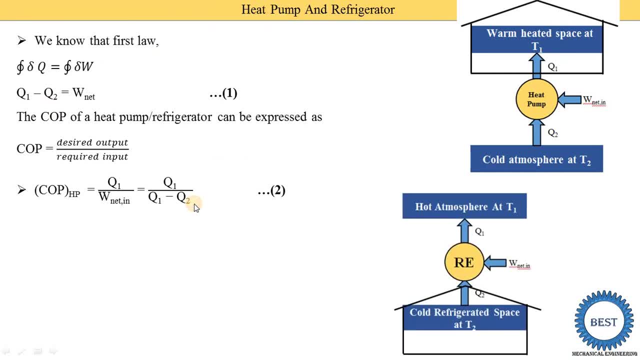 to q1 minus q2. now, next we find out the equations for the COP of refrigerators. okay, so here you see this: the diagrams of the refrigerator, functions of the refrigerator. is to the cooling, okay, and the cooling is done in this bottom part, means on a sink, okay, so here the q2 quantity of the heat is absorbed. so this: 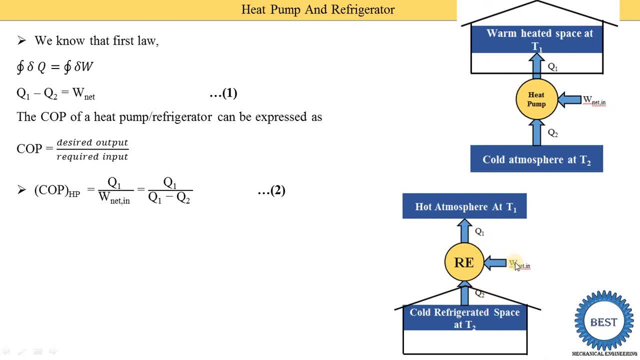 q2 is our output okay and what is the input? input is same. that is a W net, okay. so COP of refrigerator is written like this: COP bracket over R. output is the q2 okay, work input is the W net okay, and W net is also written as the q1. 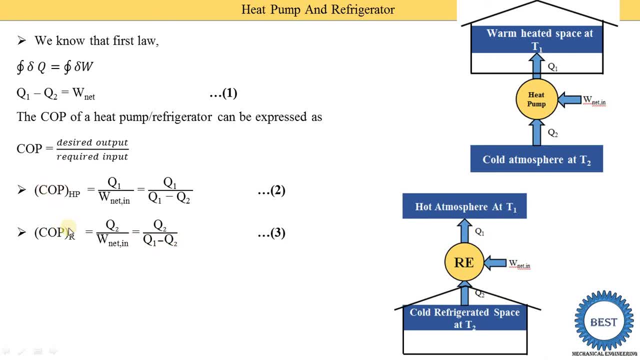 minus q2. okay, so that is a simple difference. in the COP of heat pump and refrigerator it is a q1 upon q1 minus q2. COP of refrigerator is q2 upon q1 minus q2. now we make the one relations of the COP of heat pump and the COP of refrigerators from the equation 2 and 3.